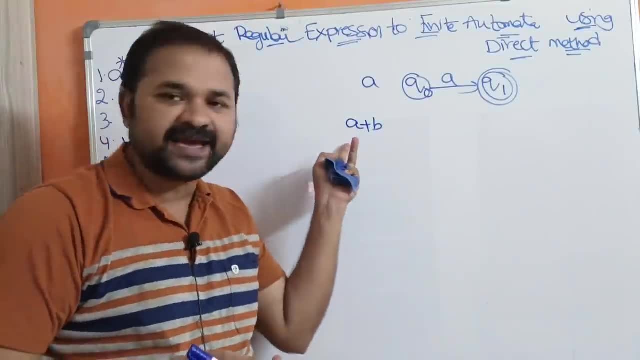 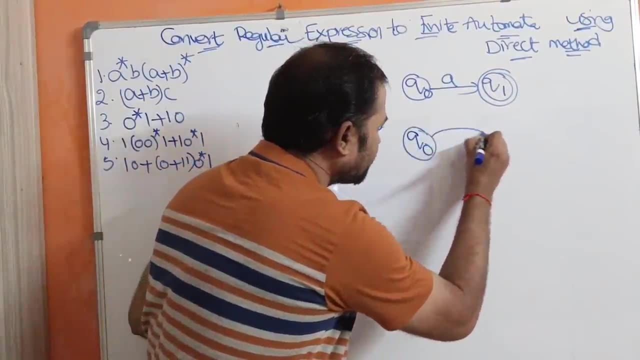 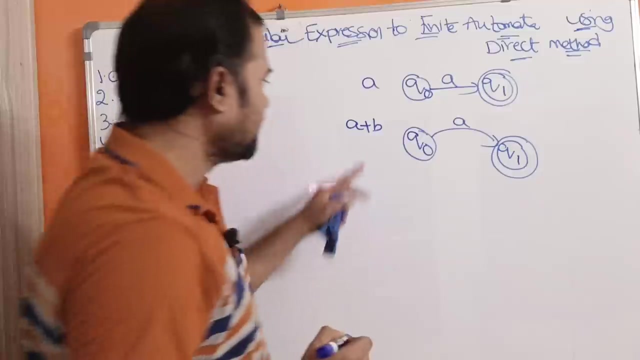 union operation. So union means it may be either A or B. So let the current state is Q0.. So Q0 on A will go to the next state. Let the next state is final state. Likewise A or B. So Q0 on B goes to the final. 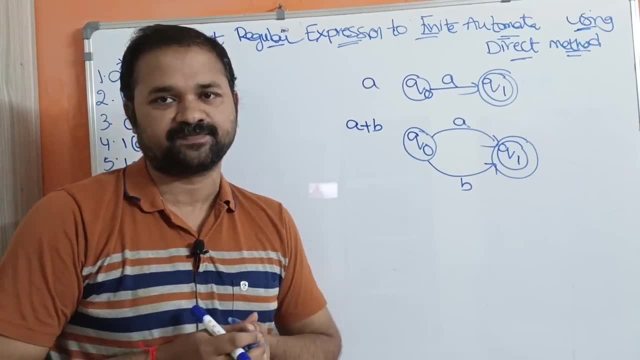 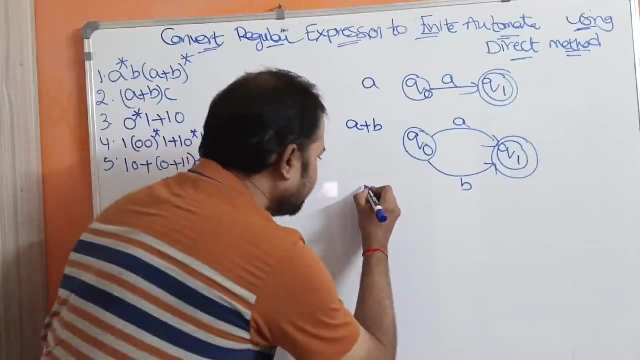 state that is Q1.. So this is about R operation. So here this is the finite automata for the regular expression A plus B. Next let the regular expression is AB, A, dot, B. So dot stands for concatenation. Here we require: 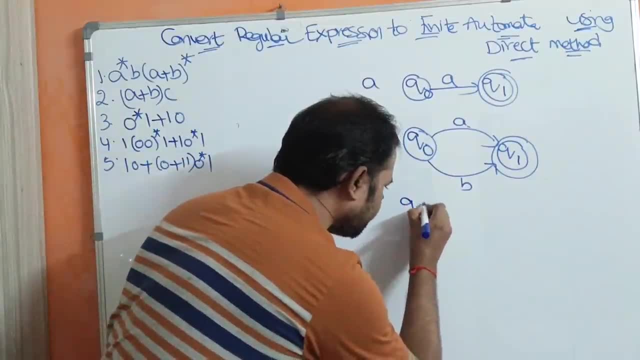 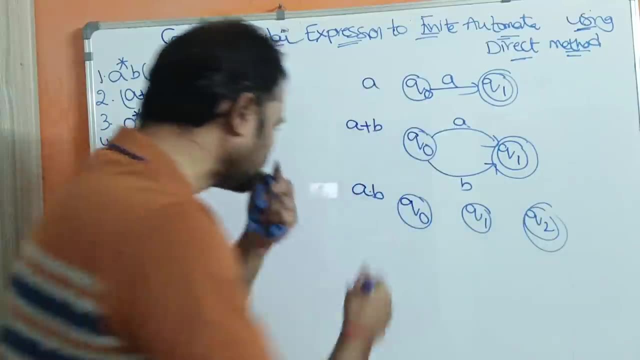 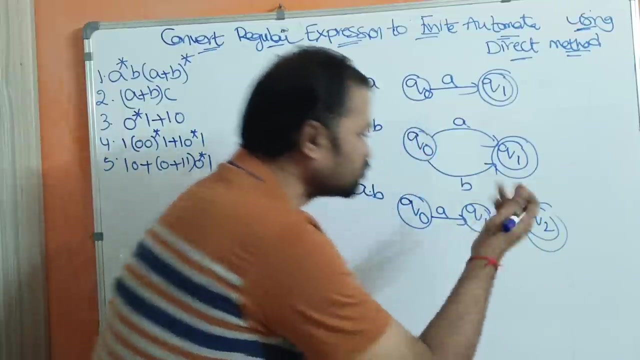 three states. So let the initial state is Q0.. Let the next state is Q1.. Let the final state is Q2.. So here the input symbols are A and B concatenation. So Q0 on A goes to Q1.. Next to Q1 on B goes to. 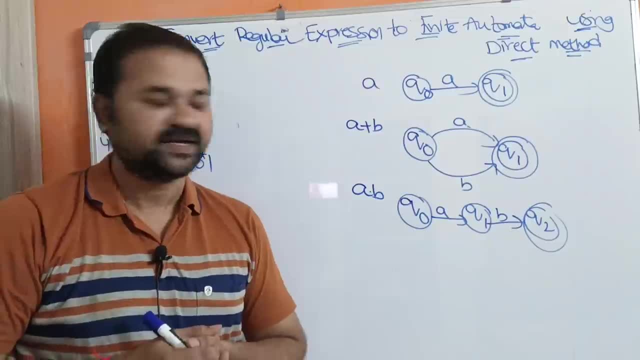 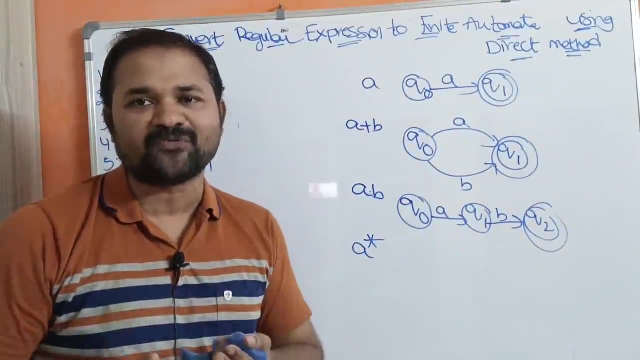 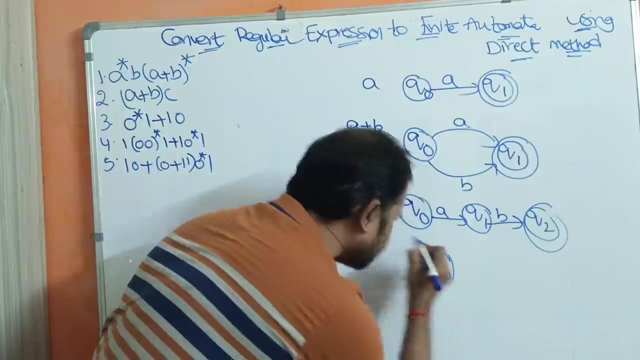 Q2.. Let Q2 is the final state here. Now let us see one more regular expression. that is A star. So star stands for clean closure. So any number of A's, including zero number of A's. So let the state is Q0 here. Let the state is: 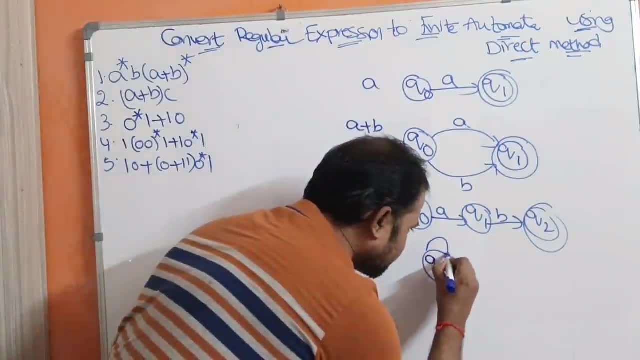 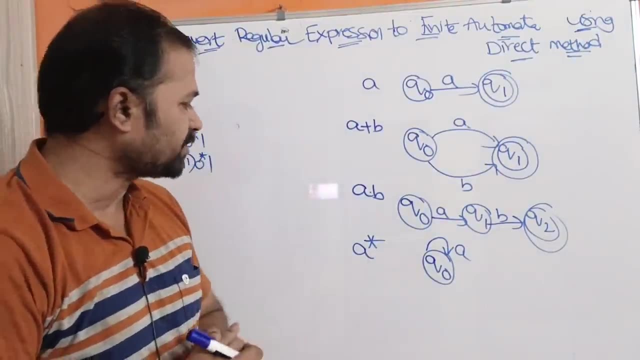 Q0 here. Here star means any number of A's, So simply we have to write as final state: Okay, Final state: This is about A star. Now let us see the next regular expression. That is A plus B whole. 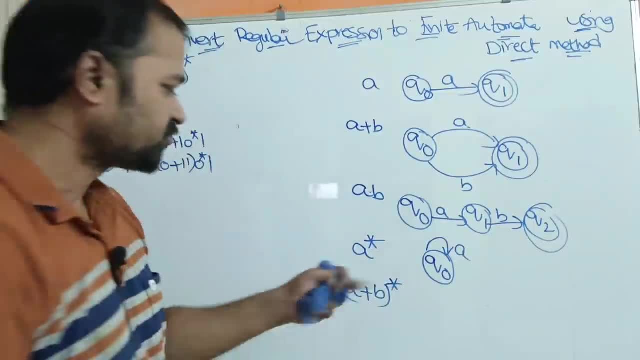 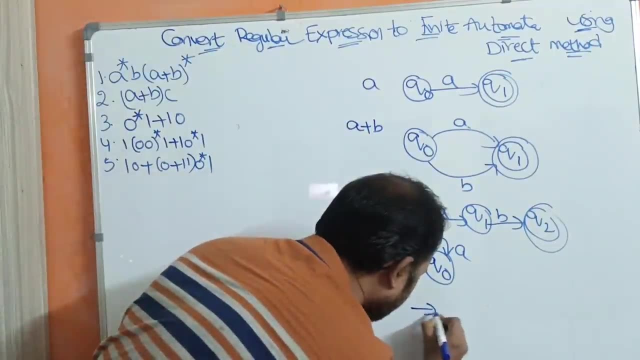 star. A plus B: whole star. So we know the meaning of A plus B. A plus B means either A or B. So simply we can write the self loop. Let the current state is Q0.. Q0. So simply we can write the self. 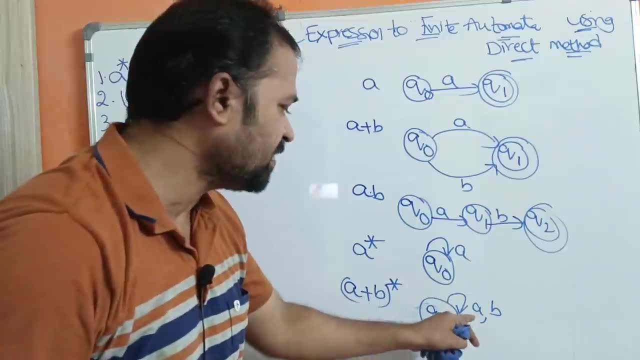 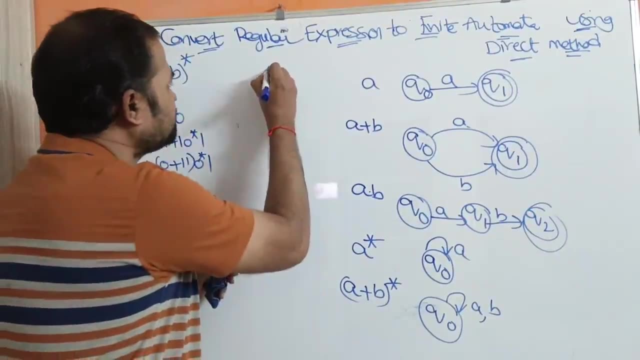 loop A comma B, A comma B, So any number of A's or any number of B's. Okay, So this is the finite automata for this regular expression. Now let us see the last simple regular expression: AB whole. 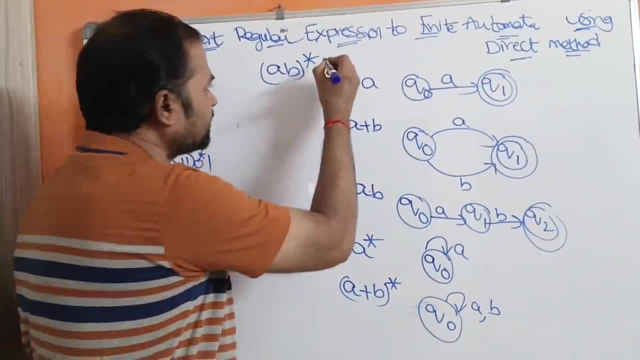 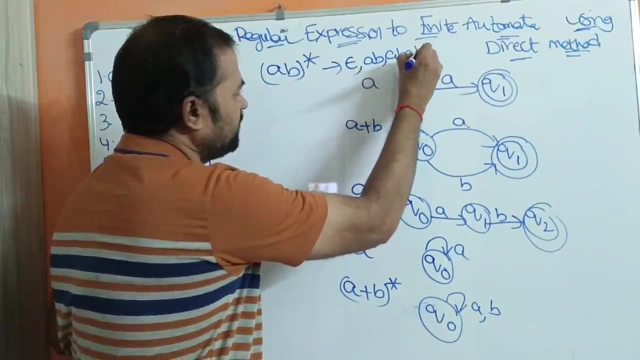 star, AB, whole star. So what is AB? whole star. So zero number of A's and B's means epsilon. So 1AB means AB, Next to 2AB means AB, AB, likewise. Okay. So let the current state is Q0.. Q0.. Let the 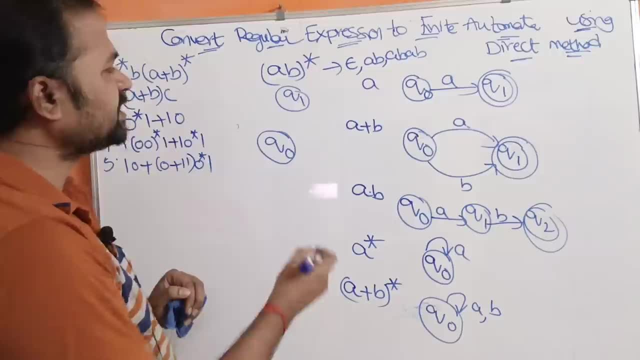 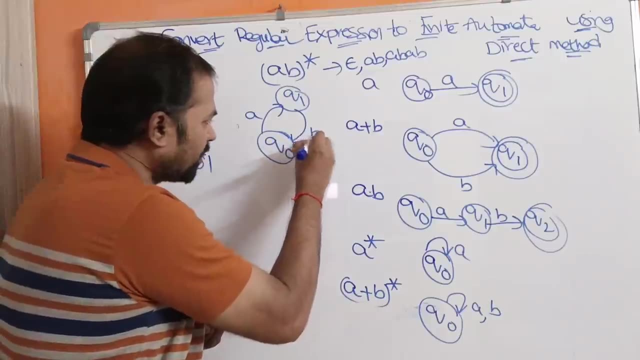 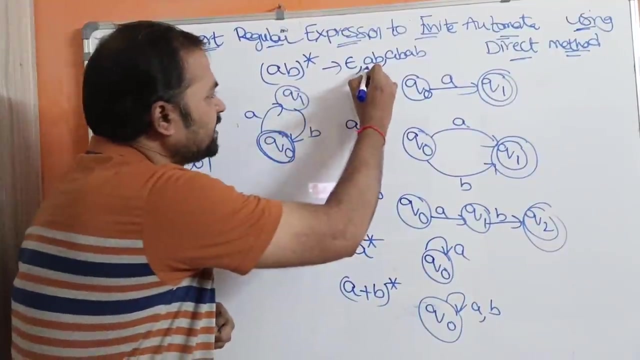 state is Q1.. Next here, what is the regular expression? AB? So Q0 on A goes to Q1.. Next to Q1 on B goes to Q0.. Here Q0 is the final state. Q0 is the final state. Okay, So let us assume that the regular expression is epsilon: Epsilon. 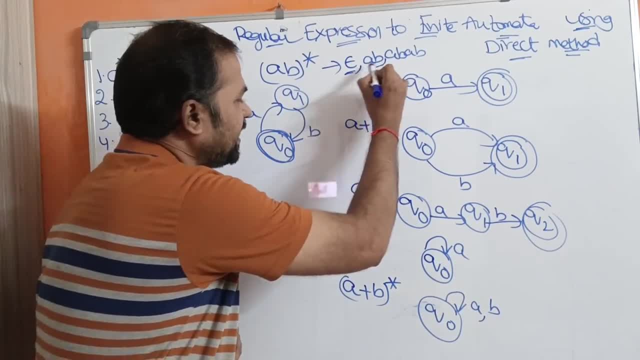 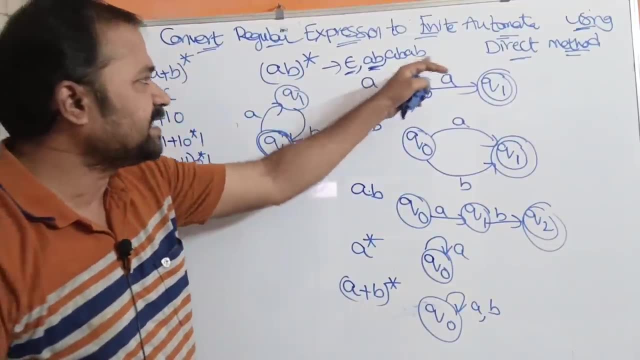 means we will be at Q0 only. Next let the expression is AB. AB means Q0 on A goes to Q1.. Next to Q1 on B goes to Q0.. Let the string is AB, AB. So A next to B, AB. So here this Q0 is the. 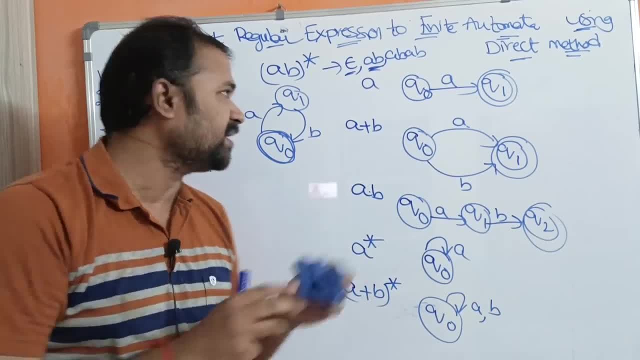 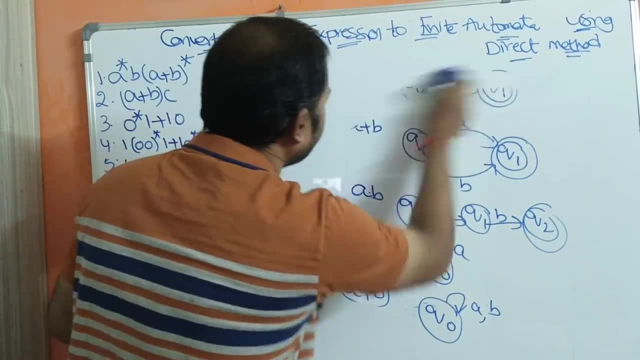 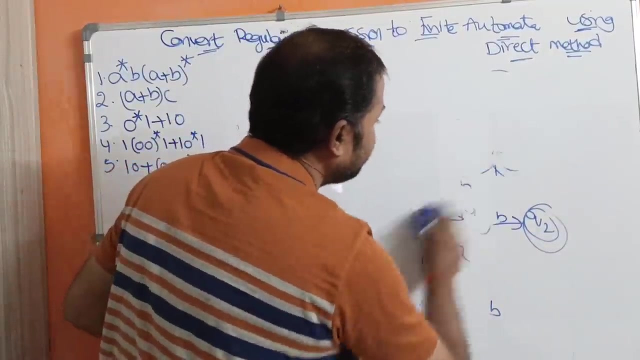 final state. Okay, So in this way, we can represent the simple regular expressions. Now, with the help of this knowledge, we need to convert these five regular expressions into the finite automata with the help of direct method. So here we are using which approach? Direct method approach. Okay, So let us see. 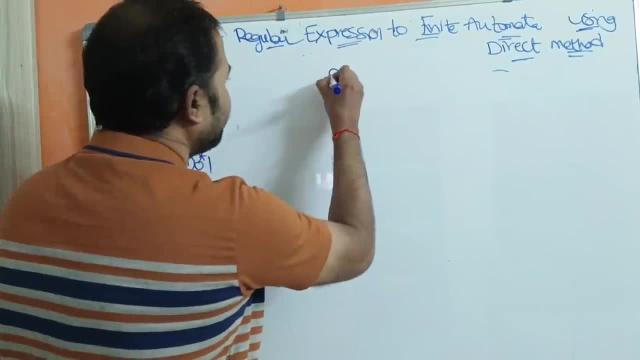 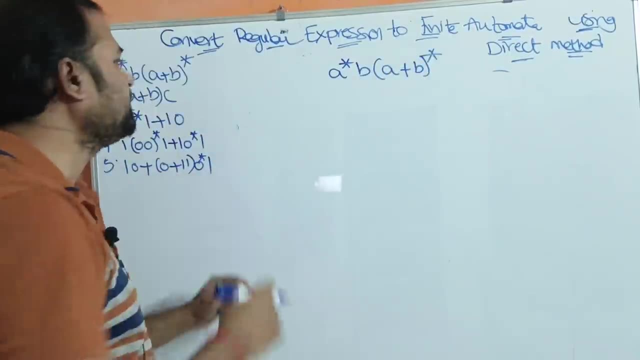 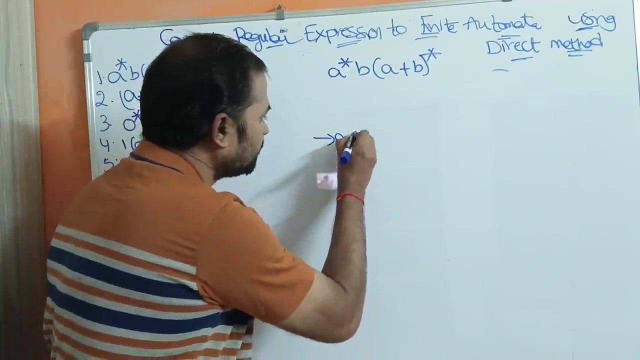 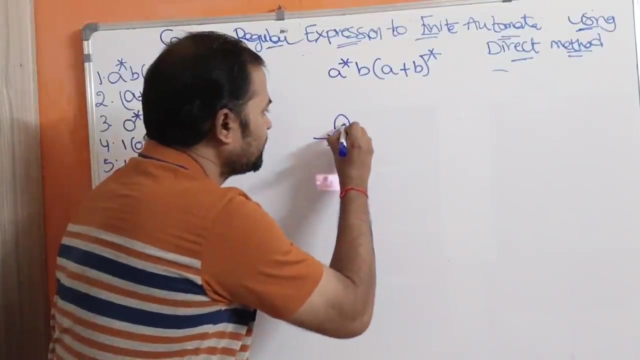 the first example. The first example is: A star B into A plus B whole star. A star B into A plus B whole star. Okay, So let the initial state is Q0.. Q0. Here, A star, A star means what? Simply we can write the self loop, Self loop. Simply we can. 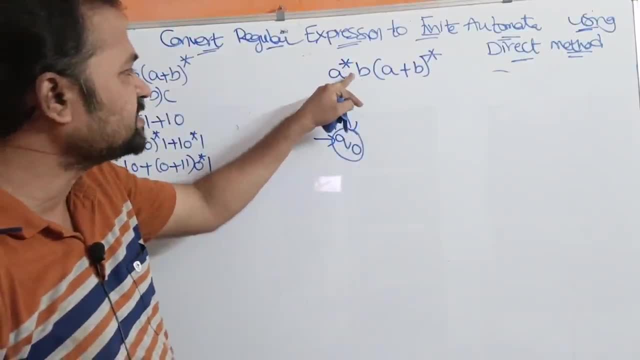 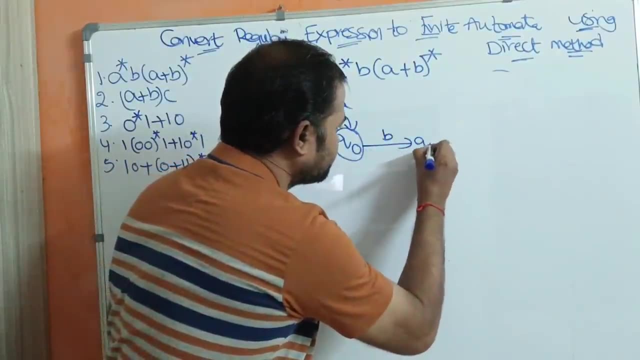 write the self loop Next next to B. So this is multiplication. So multiplication means we require one more state, So B. Next state is Q1.. So A star B is over, So A star into B Next. 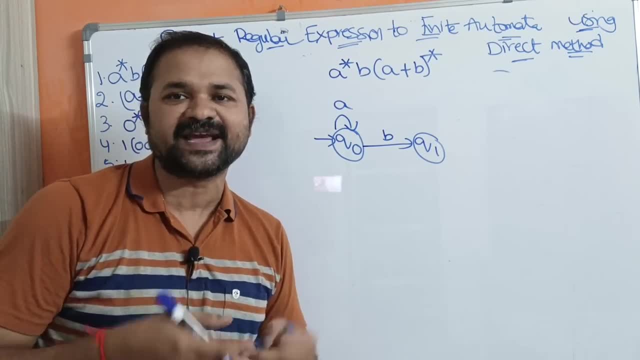 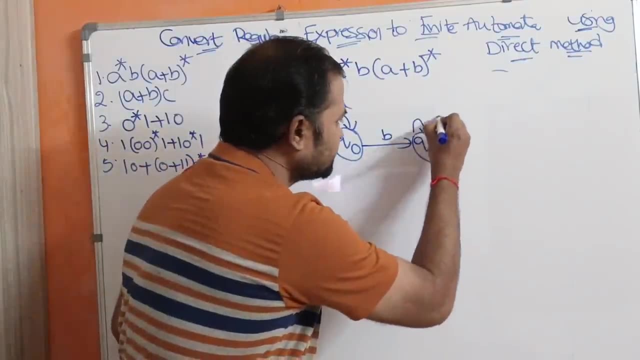 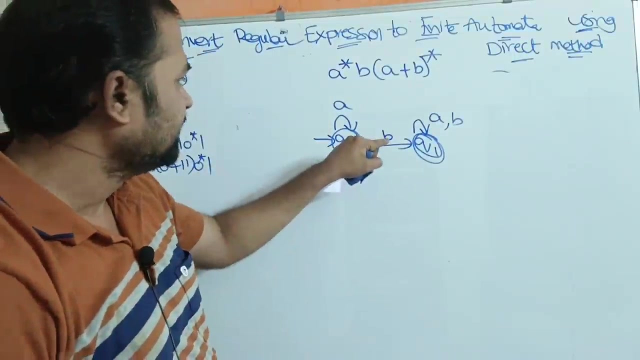 A plus B whole star. Already we have seen how to represent A plus B whole star. A plus B whole star is the final state, So this is the final state. Q1 is the final state, So this is A star. Next, 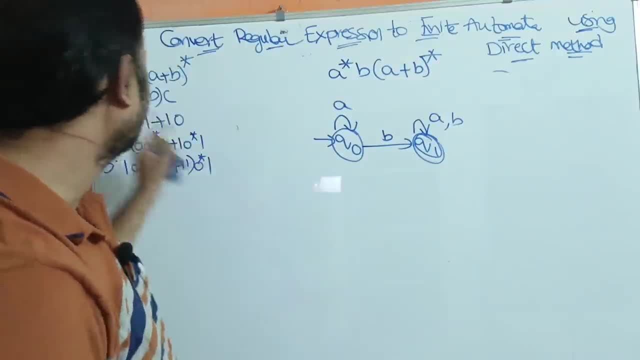 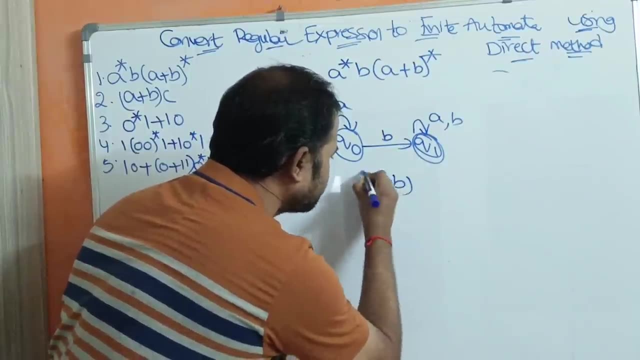 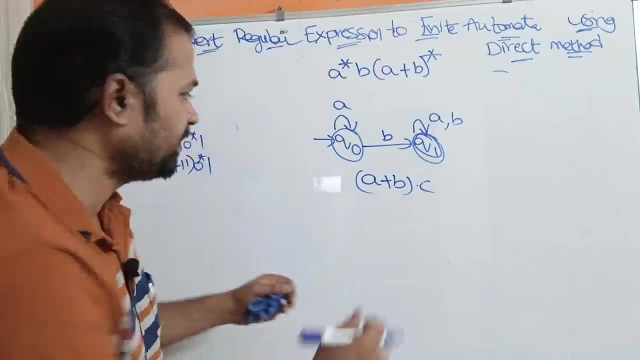 this is B. Next, this is what A plus B whole star. So this is the finite automata for this regular expression. Next example: So this is the regular expression A plus B into C: A plus B into C. Now our target is we have to convert this regular expression into the finite automata. Okay, 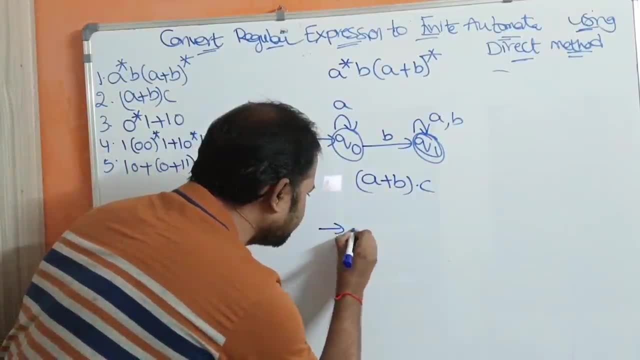 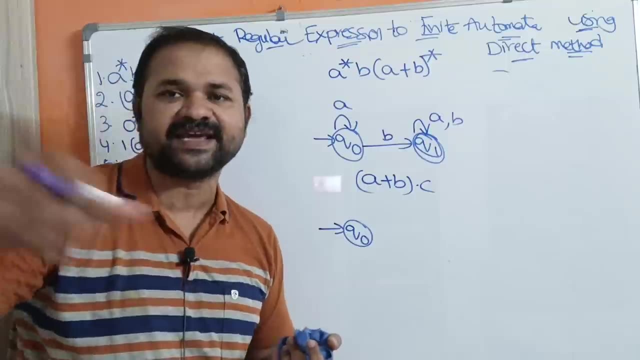 So this is nothing but concatenation. Okay, Let the initial state is Q0.. Q0.. So we know how to represent A plus B. So A plus B means either A or B. So next first Q0 on A goes to Q1.. Next. 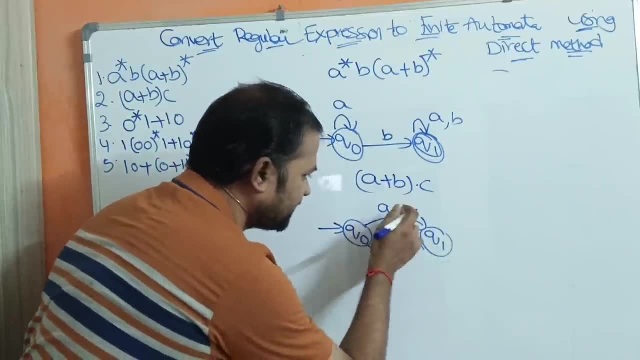 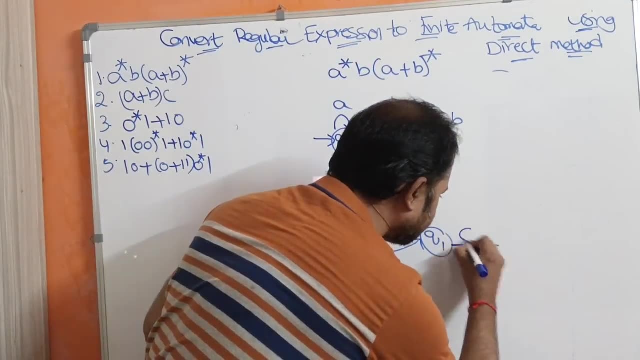 plus means R operator. So this is nothing but R. Okay, It may be either A or B, So A plus B. Next into means: we require one more state, So we need to apply C on Q1.. Let it be the final state. 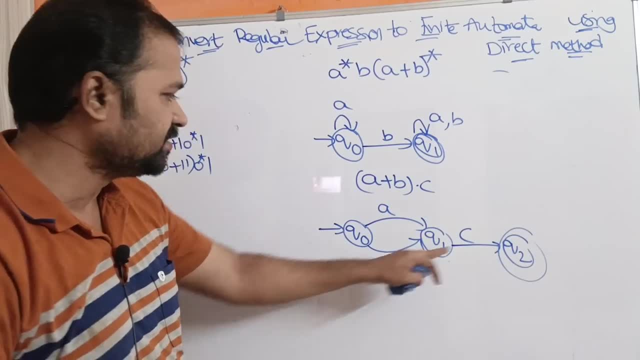 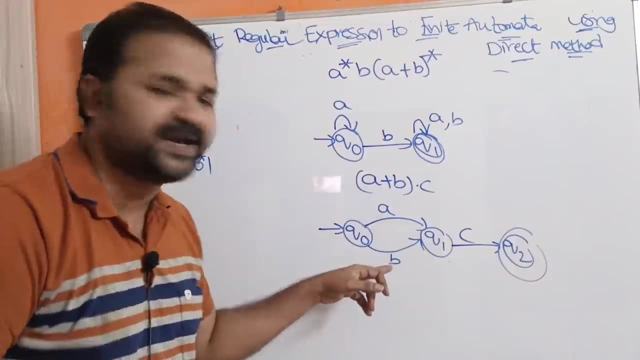 So this is nothing but A plus B into C. So this is the finite automata for this expression. So if we consider here: on Q0, only A and B are used, C is not used. On Q1, only C is used, A and. 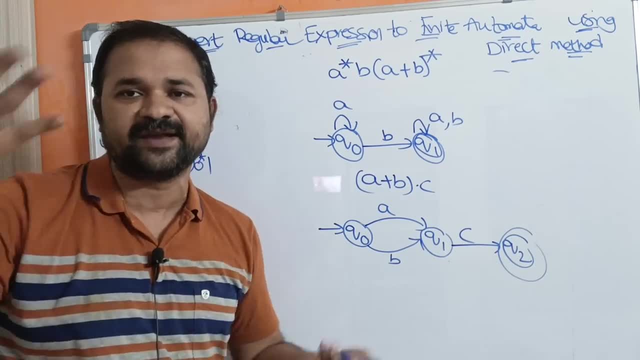 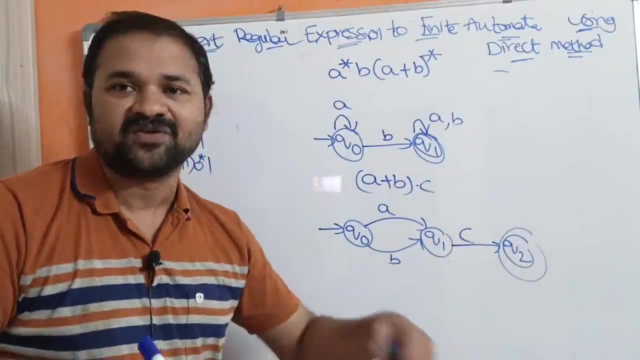 B are not used. So if the question is given for more marks, like 10 marks, then it is better to convert this DFA into the NFA. Okay, This NFA into the DFA. Why? Because what is NFA? NFA means 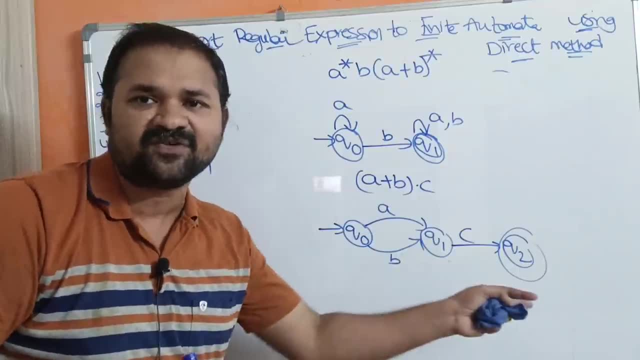 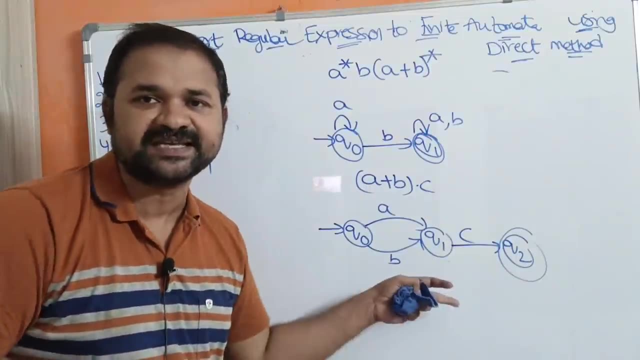 we may use either, If here the input alphabet contains three symbols, But on state Q0, only two symbols are used. On Q1, only one symbol is used. So this is NFA. So we have to convert this NFA into DFA. 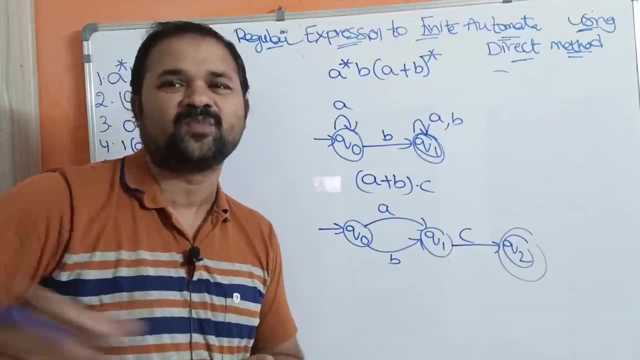 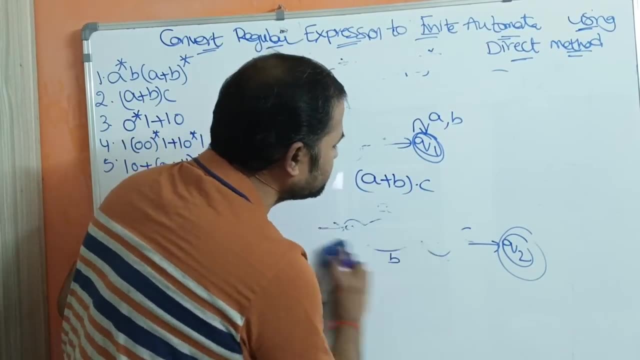 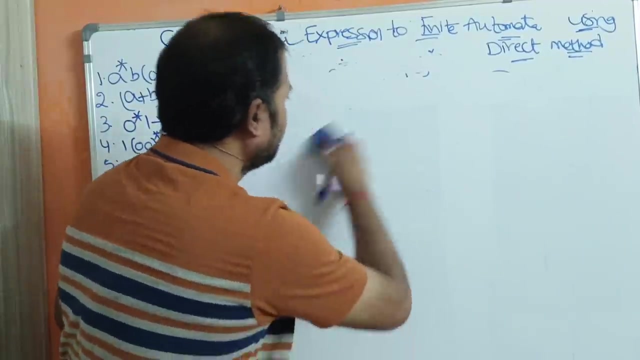 But 99 percent. the question will be given for three to four marks only. Why? Because these are the simple expressions. Suppose if the question is for more marks, then it is better to convert NFA into the DFA also. Already we have seen that in the first unit. I will share that link in the 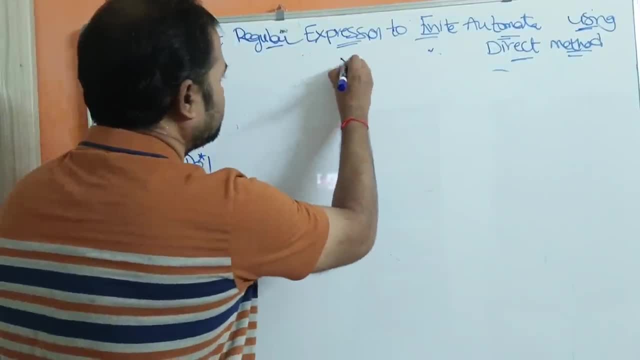 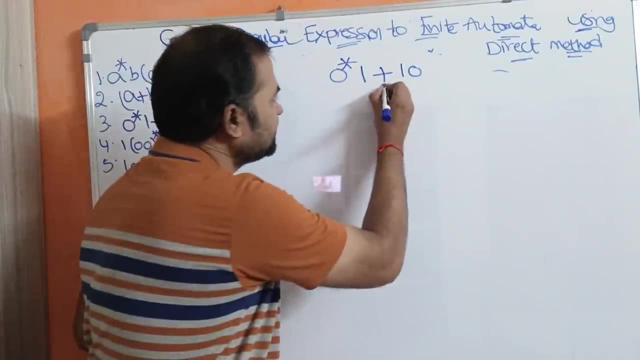 description. Next, third regular expression: 0 star 1 plus 1: 0.. 0 star 1 plus 1: 0.. So this is nothing but what Plus operator, Union operator. So let the initial state is Q0.. So if you want, 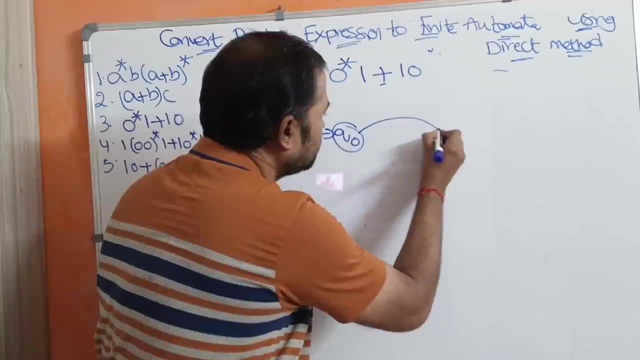 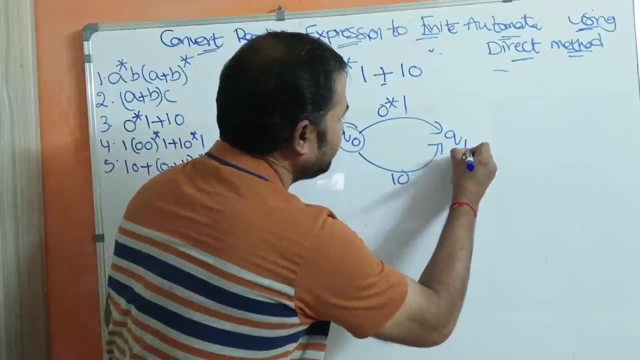 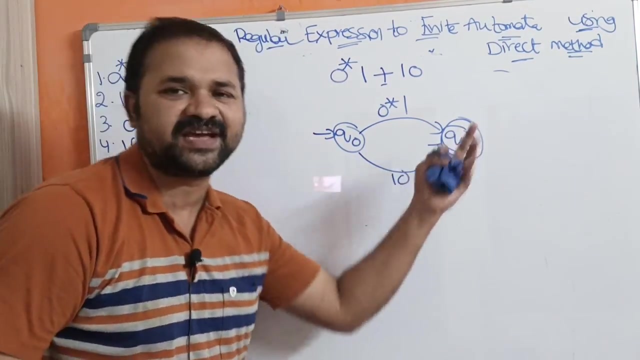 we can elaborate in detail. So this is nothing but 0, star 1.. And next R means either this one or this one. Okay, Next, let the state is: Let the state number is QF, So QF specifies that it is the final state. Okay, If you want, we can give the state number. 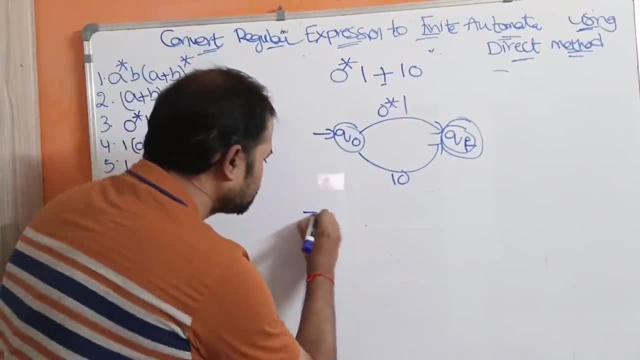 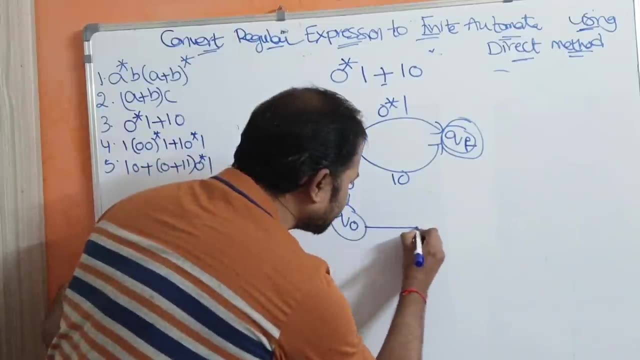 also, There is no problem. Next one is 0 star- 1.. So 0 star means we know how to write 0 star. It is self-loop. So 0 star into 1. So into means concatenation. Next, what is the final state here? 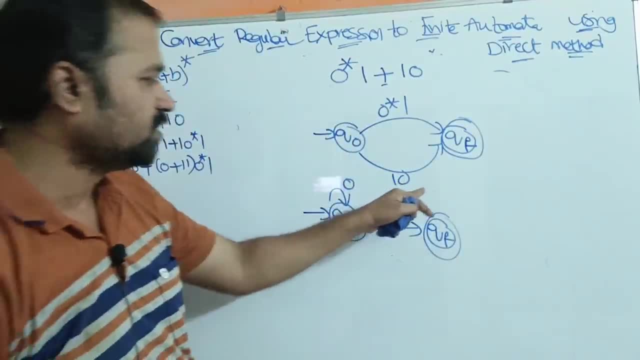 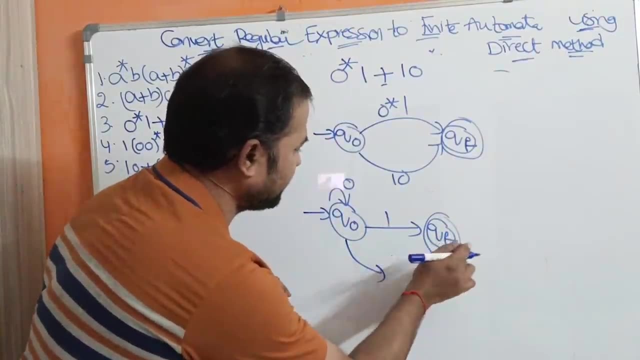 QF is the final state. Next year we have 1: 0.. So how to write 1: 0?? So for 1: 0, we require two more states. Okay, One state is enough Already. we have that second state, So we have. 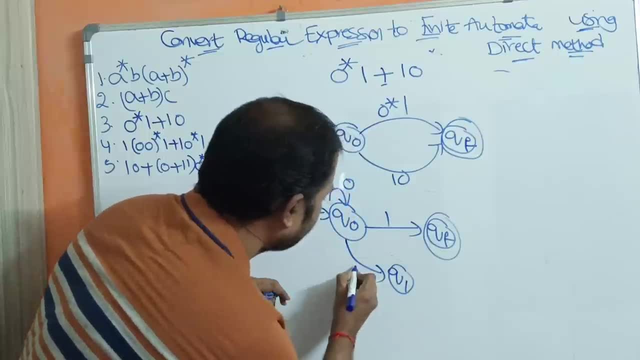 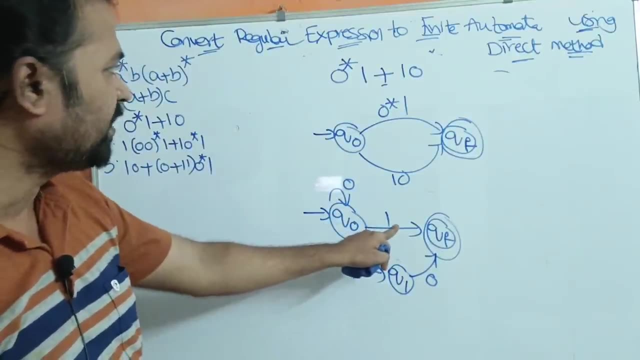 the second state. So let the next state is Q1.. So here the input is 1.. Here the input is 0.. So Q0, this is nothing but 0, star into 1 plus 1, 0.. Okay, If you want, here we can. 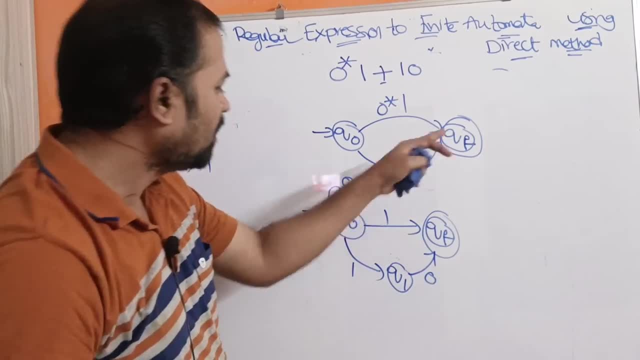 write it as Q2.. So in place of QF we can write Q2.. Or here we can write Q1.. Here we can write Q2.. There is no problem? Okay, So this is the finite automata for this regular. 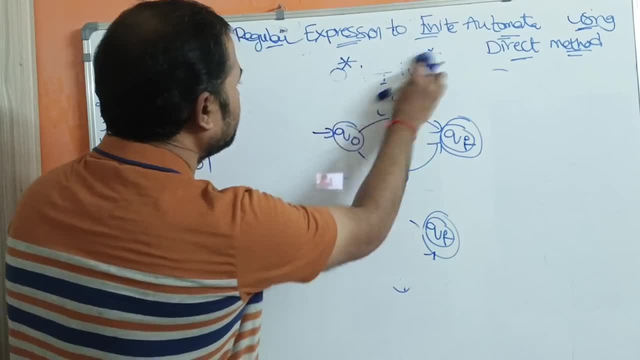 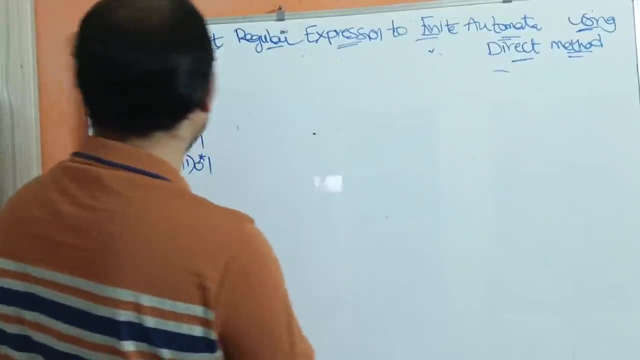 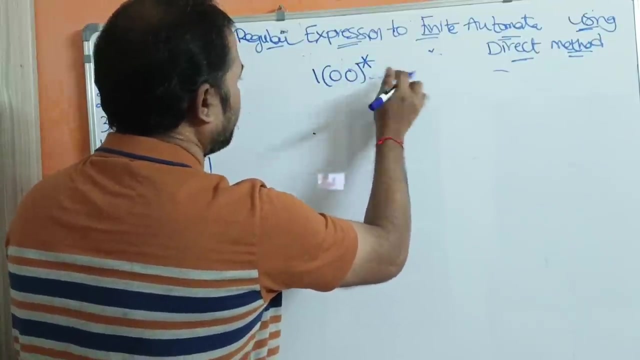 expression. Now let us see the next example. So what is the next example? So 1 into 1 into. So this: 1 into 0, 0 star, 0, 0 whole star into 1 into 1 plus 1, 0 star, 1, 0 star. 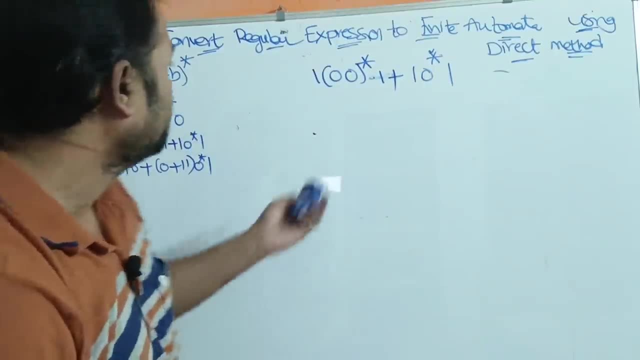 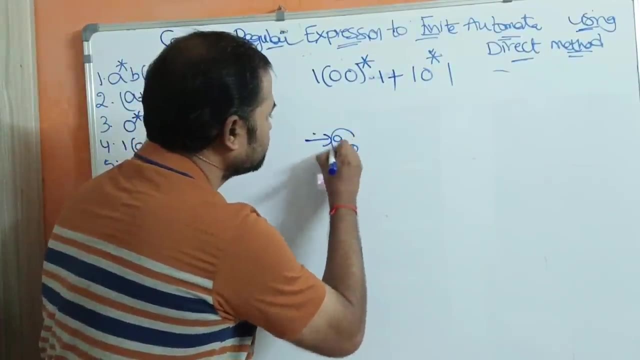 1. So 1 into 0, 0 star into 1 plus 1, 0 star, 1. Okay, So now let us write the regular expression here. So this is nothing but what R operator, So R operator means we may have. 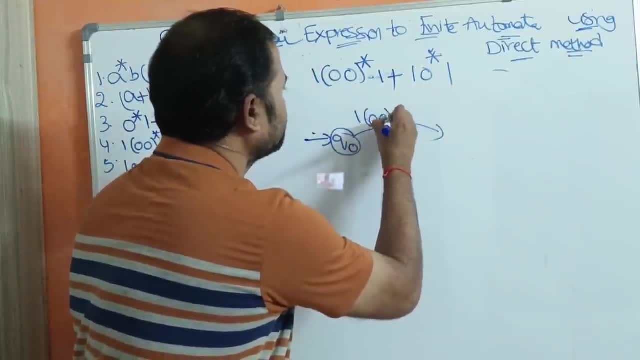 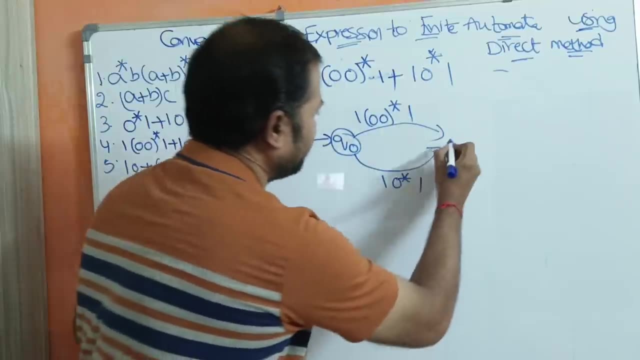 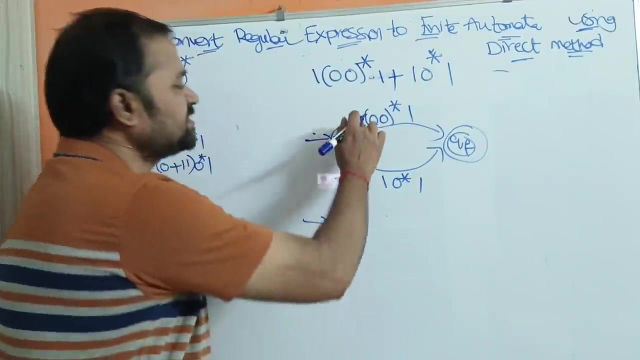 either this situation, So 1 into 0, 0 star into 1.. Next, 1: 0 star 1.. It may be either this one or this one. Let the final state is QF. Okay, Next Q0.. Next 1 means this is nothing but concatenation. 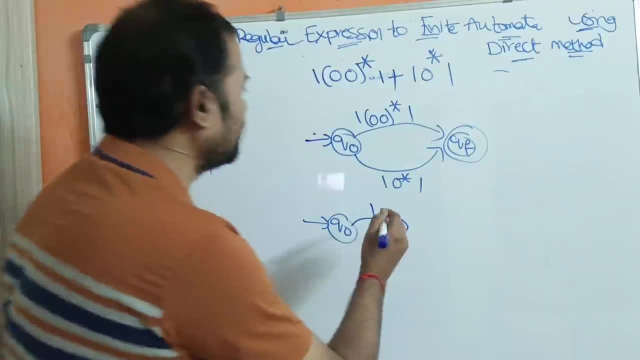 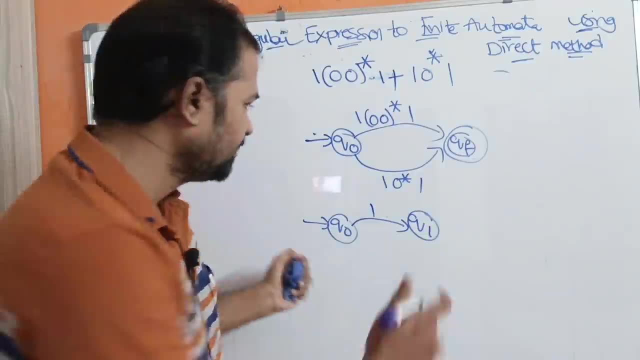 operator. So if we apply 1 on Q0, then we will go to the Q1 state Next year. we have 0, 0 star, So we know how to write 0, 0 star. Okay. So let us take one more state here. 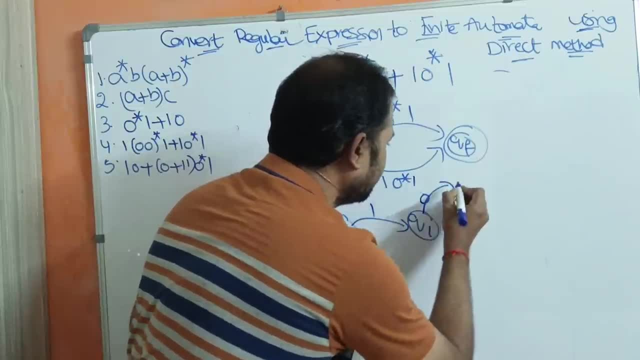 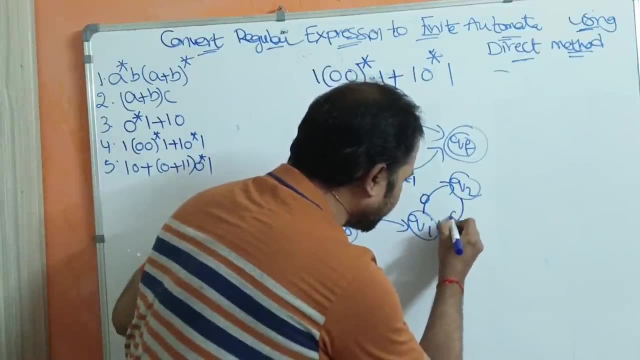 So 0. So here let us write here, Let the state number is Q2.. So Q1 on Q2.. Q1 on 0 goes to Q2.. Next, Q2 on 0 goes to Q1.. Q2 on 0 goes to Q1. Okay, So 0, 0.. 0, 0. Okay, Next one. 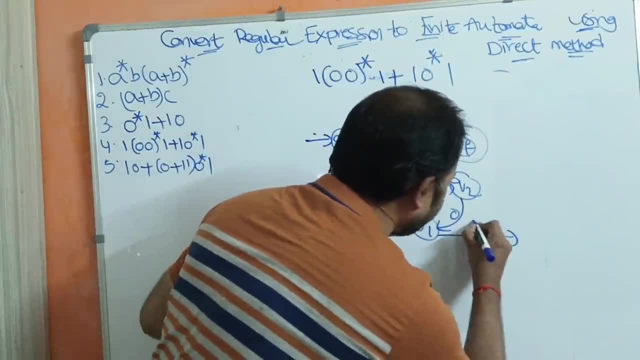 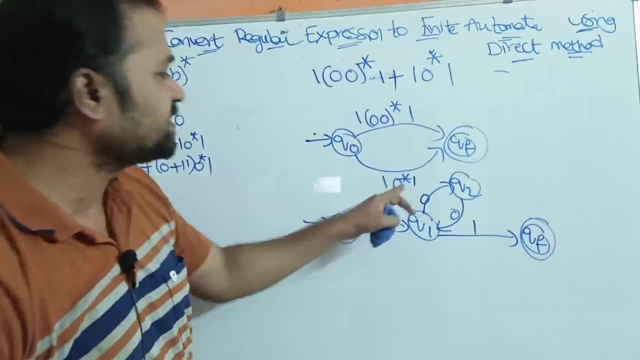 0, 0 star is over, Next one is 1.. Next one is 1.. So, on applying 1,, this will lead us to the final state, So QF. Next one is 1, 0 star. So this is also concatenation operator. So Q0 on 1 goes to the next state, That is. 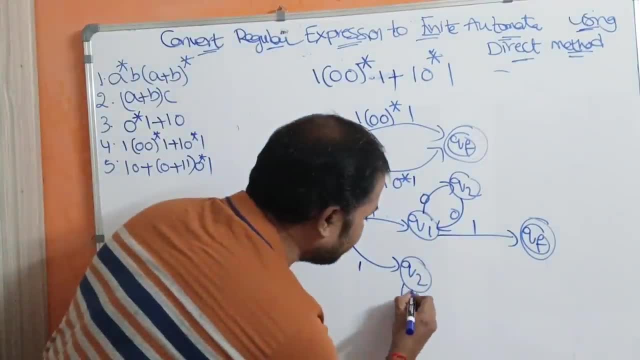 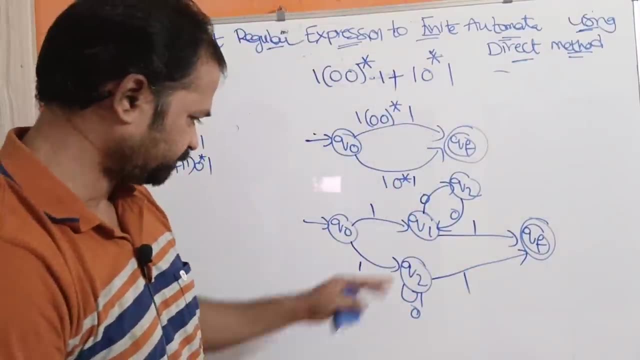 Q2.. Next, 0 star means simply we can write the cell through 0 star. Next year we have 1.. So if we apply 1 on Q2, then we will go to the final state. So this is the finite. 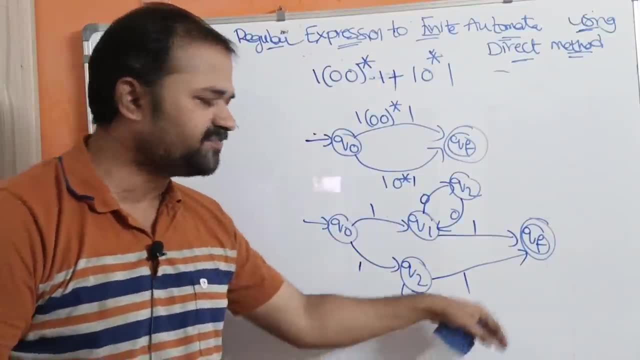 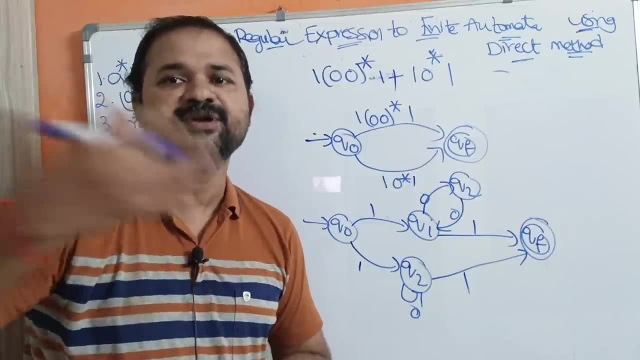 automata for this regular expression. This is DFA or NFA. This is NFA. Okay, So we can convert this NFA into the DFA by using the algorithm NFA to DFA conversion. Okay, If the question is given for more marks, like 10 marks, Suppose. if the question is given: 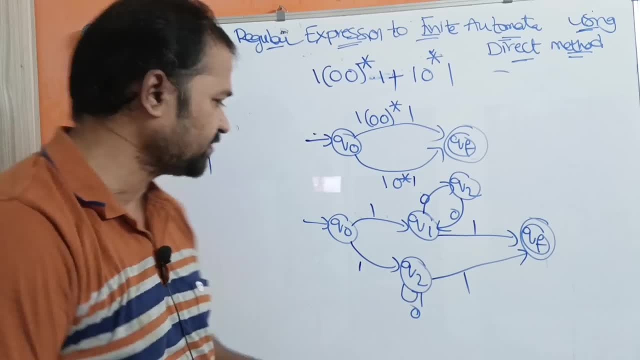 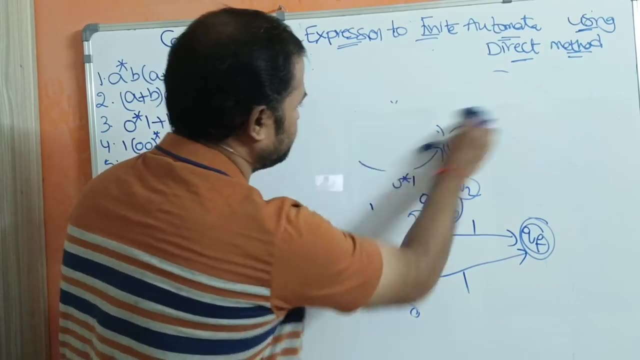 for 5 marks, then this finite automata, this NFA, is enough. Suppose if the question is given for 10 marks likewise, then it is better to convert this NFA into the DFA also. Now let us see the last example. So I will share the link in the description. So if you have 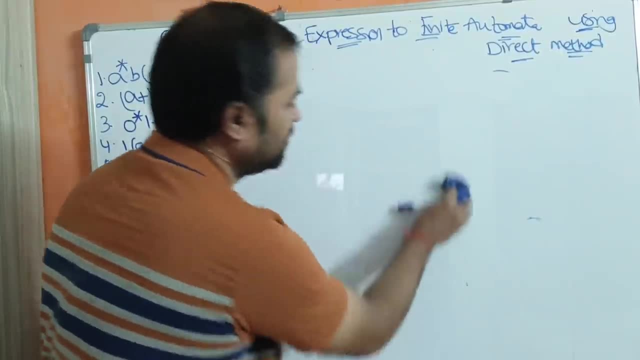 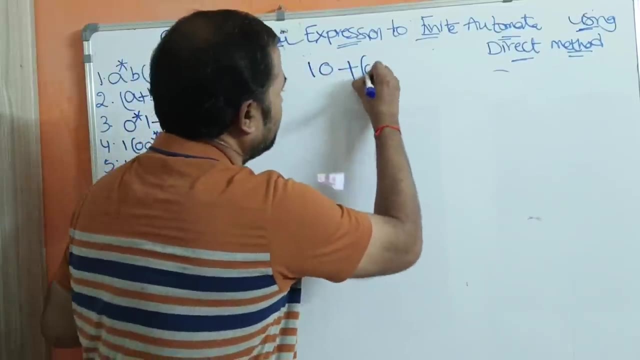 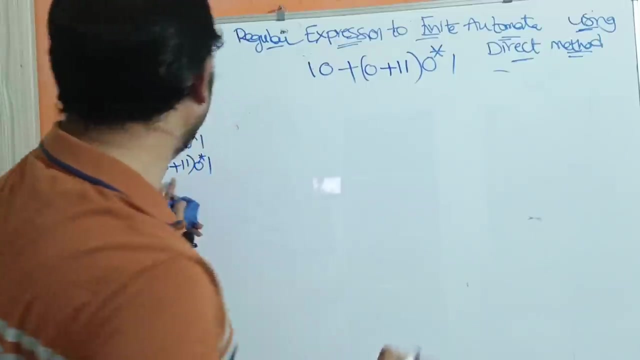 any doubt on how to convert NFA to the DFA, just please refer that video. Let us see the last example. This is most famous example. This example is given in many quotient papers. So 0 plus 1, 1, 0 star 1.. So 1, 0 plus 0 plus. 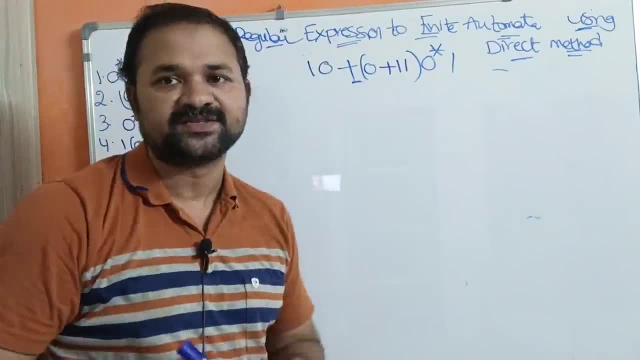 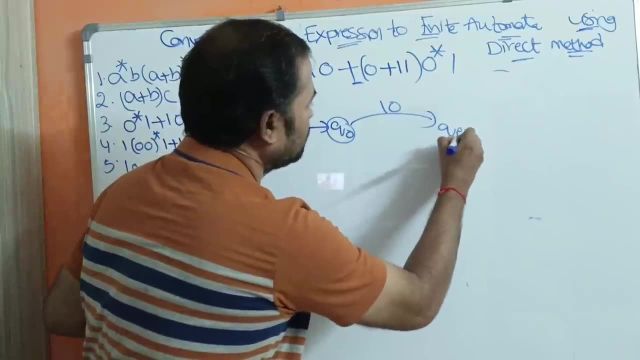 1, 1, 0 star 1.. So here this is nothing but plus. So plus means union operation. So let the initial state is: Q naught, So Q naught on 1: 0.. We will move to the final state Next. 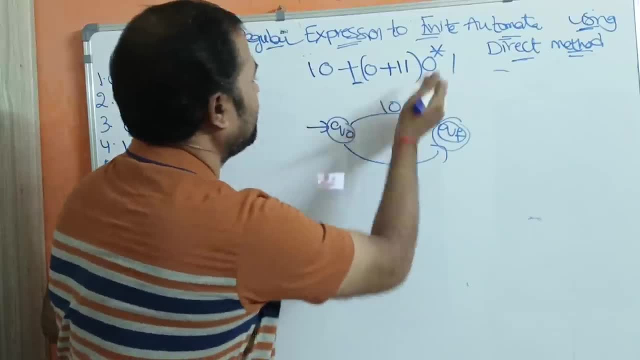 what is the second one Second after R? we have 0 plus 1, 1 into 0 star 1.. Okay, So this is the final state. Next, what is the second one Second after R? we have 0 plus 1, 1 into. 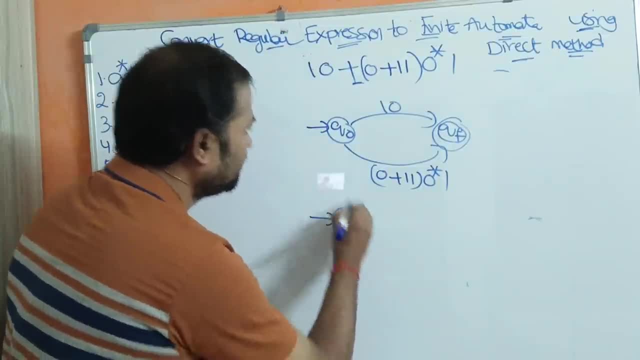 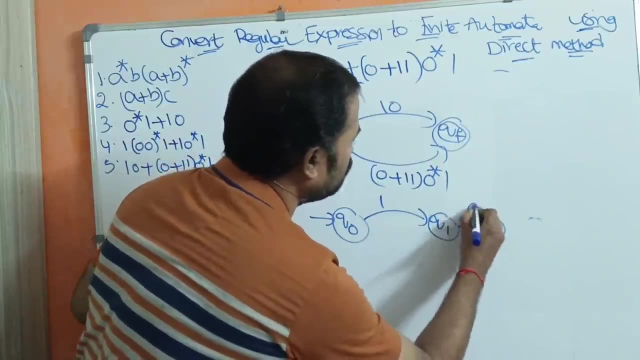 0 star 1.. Next Q naught: Next 1: 0.. This is nothing but what concatenation. So concatenation means we require one more state here. Next Q: 1 on 0 goes to the final state. Final state. 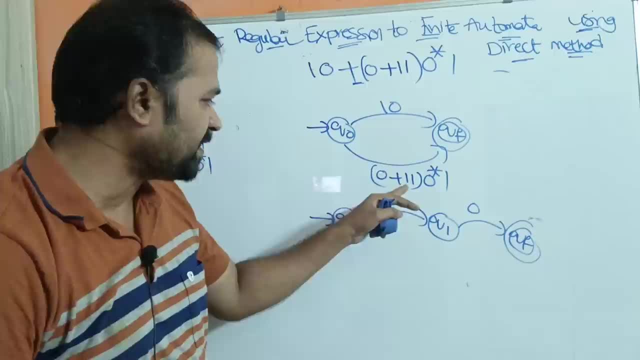 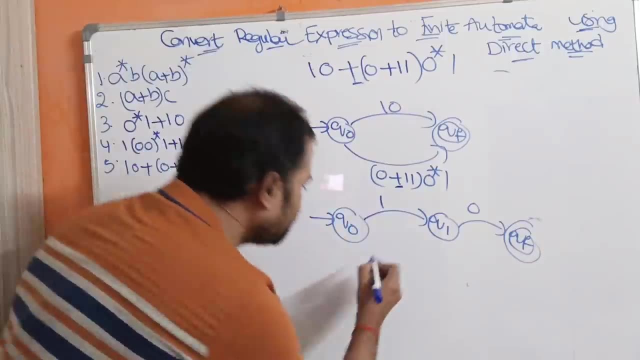 Next 0 plus 1, 1 into 0 star 1.. So 0 plus. Here we have R operator. So R operator means it may be either 0 or 1, 1. So we need to have one more state. Let that state is Q 2.. 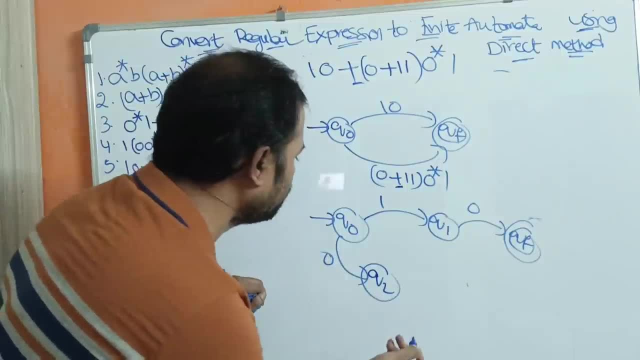 So Q naught on Q 2.. Q naught on 0 goes to Q 1.. So Q naught on Q 2 goes to Q 1.. So Q 1.. Next let us write a little bit, Little bit down. So what is the state number? Q?